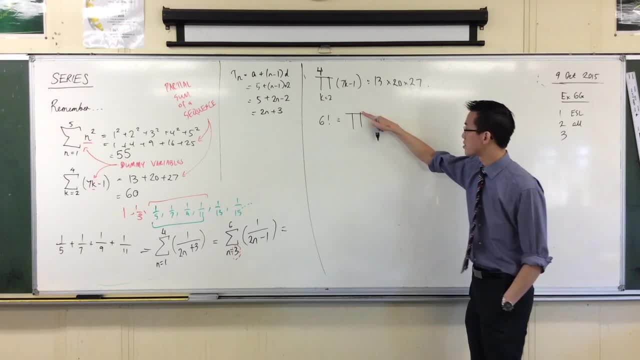 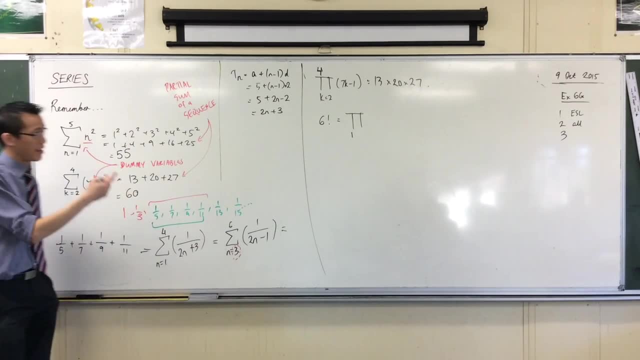 I would say okay. firstly, it's a product right. Where would you like to start? K equals 1.. Let's go ha. now be careful. right Built into both sigma and pi. it's terrible because it gets used for everything. 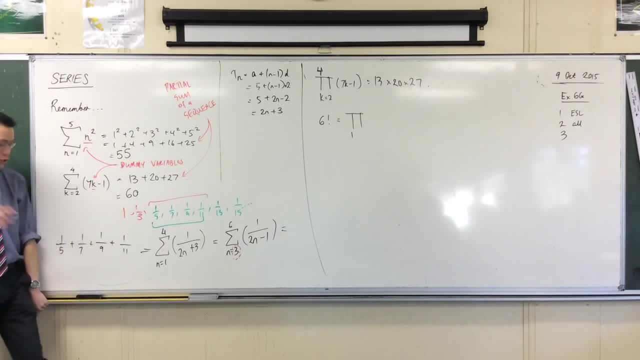 but anyway, sigma notation and that notation right is that you start from here and you go up to here. Oh, okay. Okay, Now we will get to one. What happens if you're like: well, what if I don't want to? 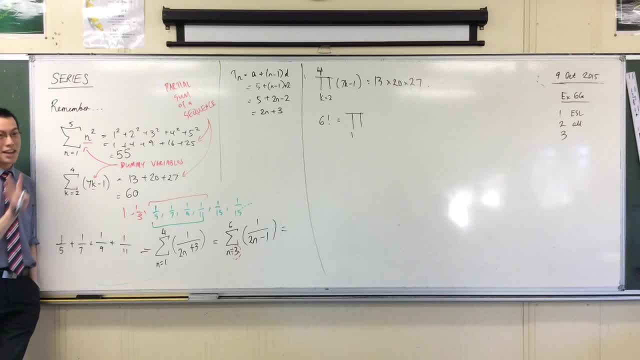 What if I want to start at 4 and end at 2?? Well, believe me, we'll get there. Okay, but for now, rather than get your wires crossed, we start at another and we increment up to get to the next one, okay? 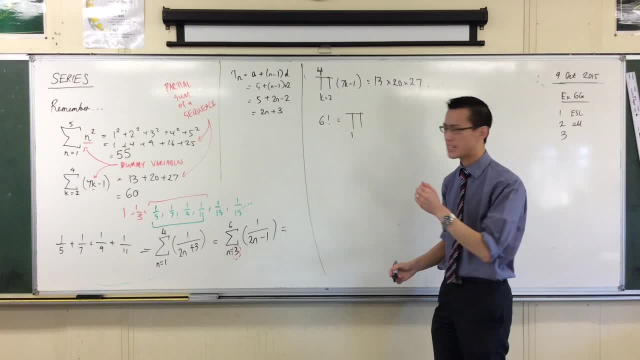 Or to get to the last one, right? Is there any point in saying k equals 1?? Is there any point to it? Yeah, because it doesn't do anything. Well, if you start from here, it tells you where to start. 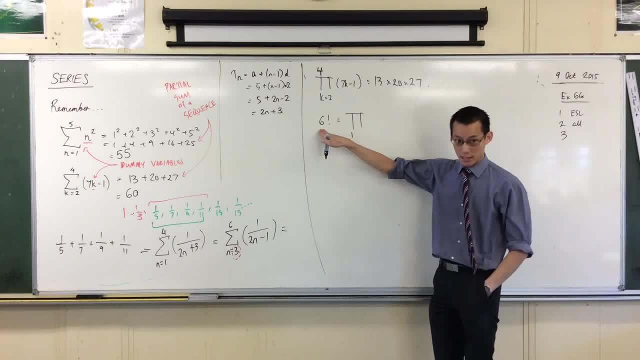 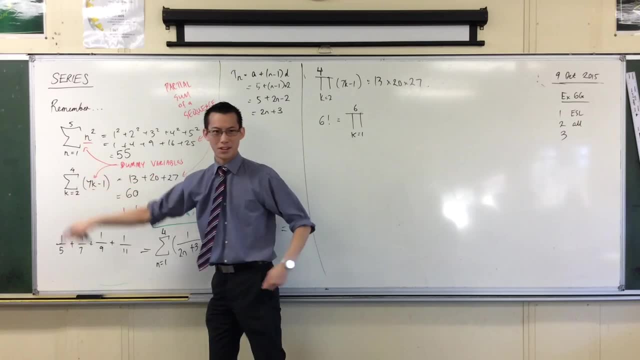 What it does help me with is, if I want 6 terms, then I can know I'm going to start at 1 and end at 6, right, Rather than, like think of some arbitrary thing where it's like I don't know where I'm going to end. 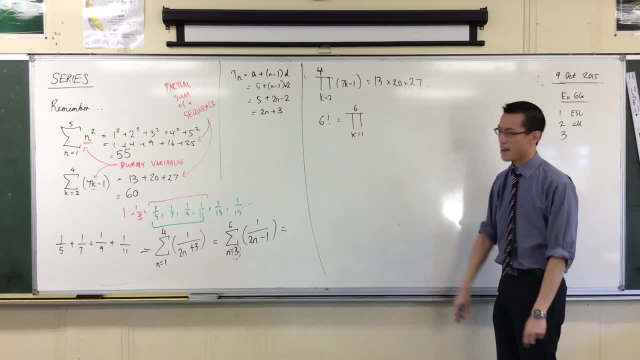 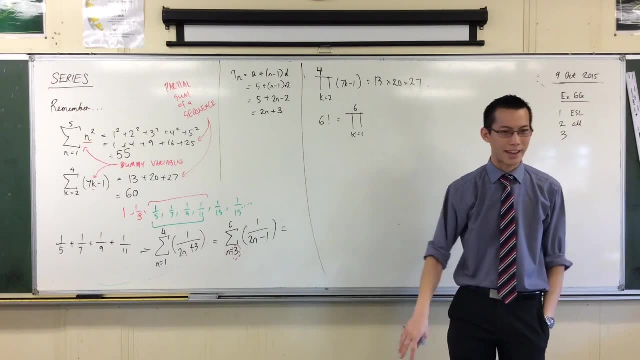 I might as well have a first term be the 1 term, okay. Now careful with this right, Because you know what 6 factorial is equal to right. It's 6 by 5 by 4, by 3, by 2 by 1, okay. 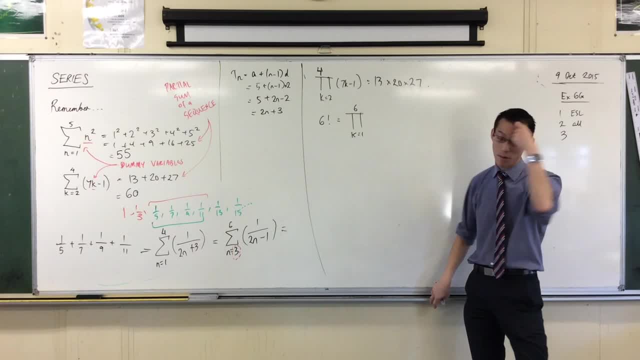 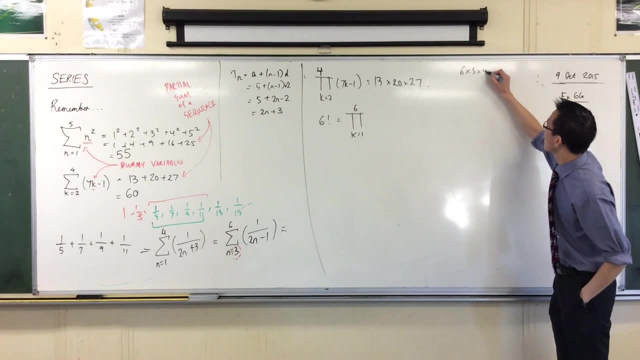 You can count. okay, Now I could write this in reverse order. I could right, But let's try writing it in the right order. right? Let's try and write it so that it will come out like this rather than this, even though this would probably be. 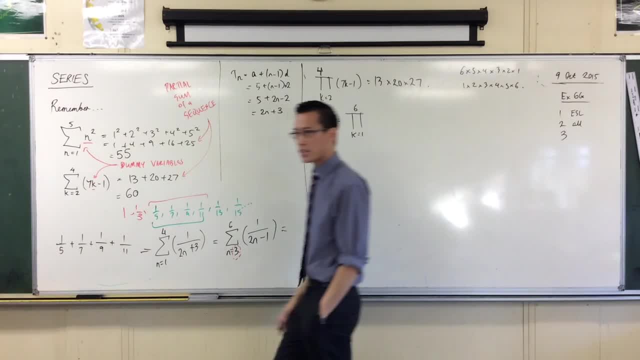 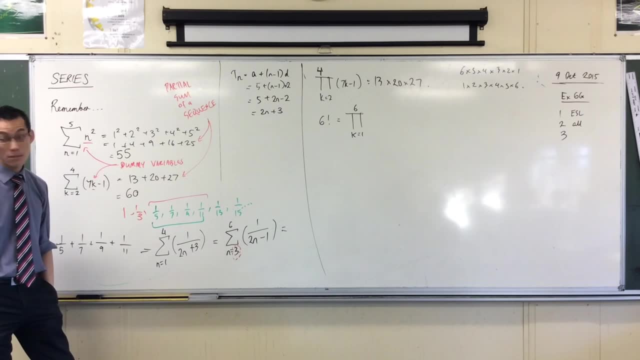 probably be easier, right? If I wanted to go down, how is this going to work? 6, 4, 6, 7 minus. oh, negative, 7 minus. So let's think about this. Let's think about this, right. 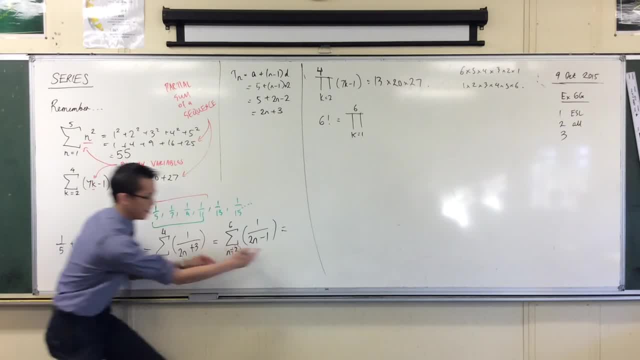 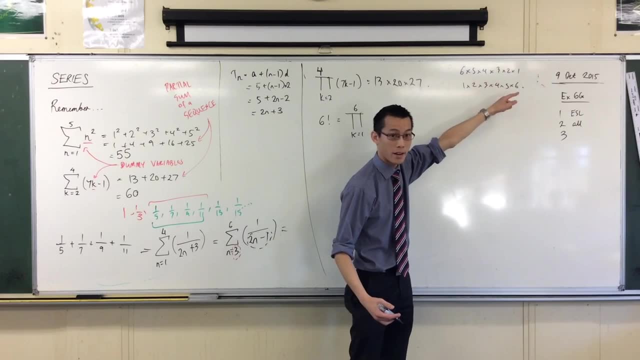 Just like. just like in this case, and in this case right, these numbers form an AP. right They form an AP: 6, 5, 4, 3, 2, 1.. 1, 2, 3, 4, 5, 6 also forms an AP, but it's a different AP.